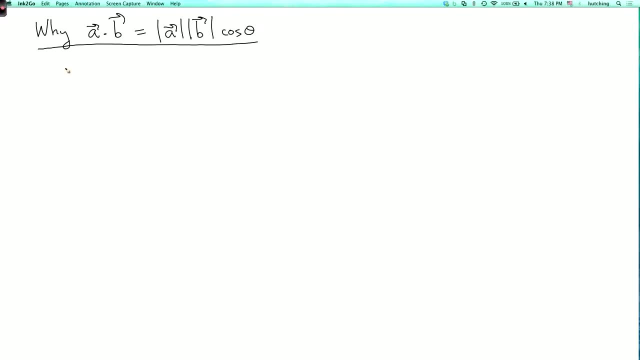 I'm now going to explain the geometric interpretation of dot product, that is, a. dot b is equal to the length of a times the length of b times the cosine of theta, where theta is the angle between the two vectors. Now let's assume that the vectors a and b are both not zero. Otherwise the dot product is zero, and this is not very interesting. 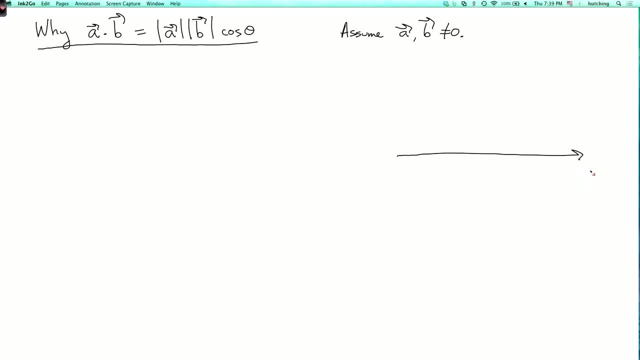 Now let's draw a picture. So here's the vector a And here's the vector b, And this angle, here is the angle theta. Now, the first step is: I'm going to drop a perpendicular from b to a like this. What I mean more precisely is the following: 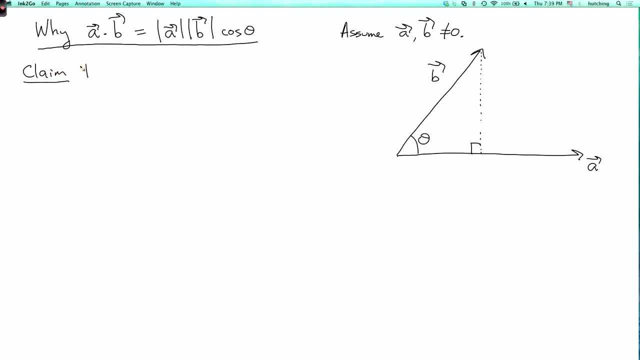 I claim that there is a unique scalar, c, such that b is equal to b. b minus c times a is perpendicular to a. So in the picture here, this piece of a, this is c times a, And then this dotted line. if I make it into a vector going up in the picture, then this vector is b minus ca. 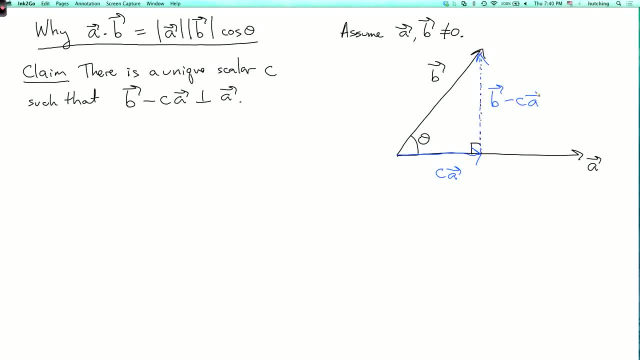 And I want this vector to be perpendicular to a. So I claim there's a unique c that makes that work. So the proof of this claim is: let's solve for c. So I have b minus ca. dot a equals zero. That's what it means for these two vectors to be perpendicular. 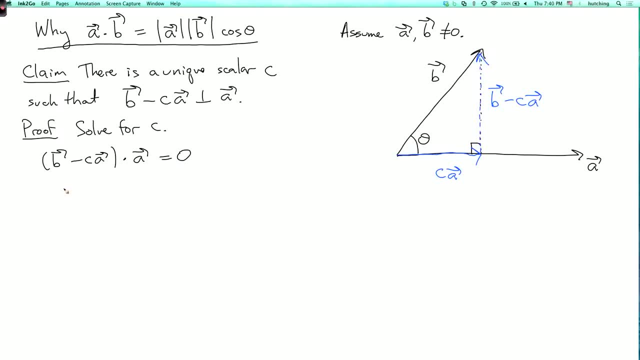 And I can expand this dot product using the distributive property. So I get b dot a a a a a a minus caa equals 0.. And I can pull the c out So I can rewrite this as b dot a minus c times a dot a equals 0. 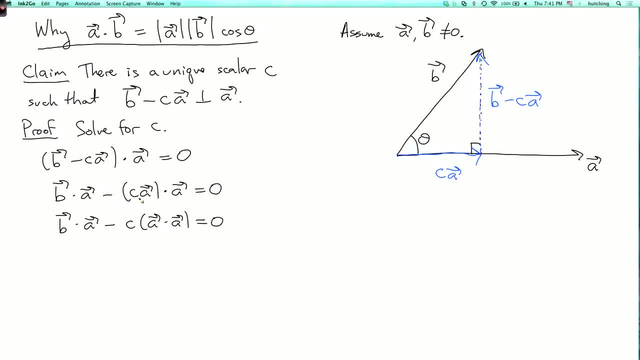 So I didn't prove that you can pull a scalar out like this, But you can check that it works, because here I just multiply every component by c. So when I take the dot product It's just going to multiply the whole dot product by c. 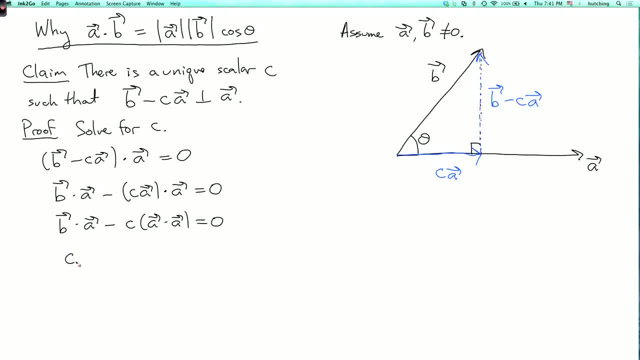 Okay, so now I can solve for c, and I have: c equals b dot a divided by a dot a, and that's just the length of a squared. so I'll write it as length of a squared And this is well defined. 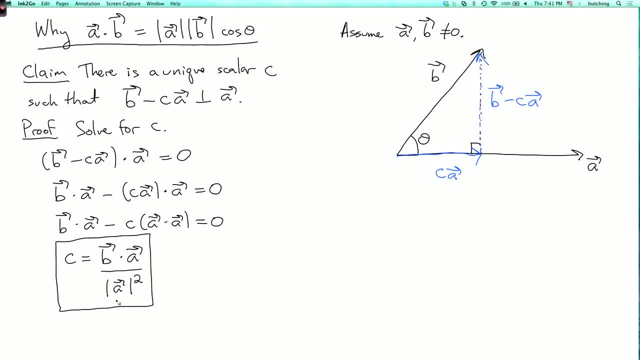 I'm not dividing by 0, because a is not 0, and so its length squared is not 0.. It's a sum of squares and they're not all 0.. All right now, what does that have to do with the cosine of theta? 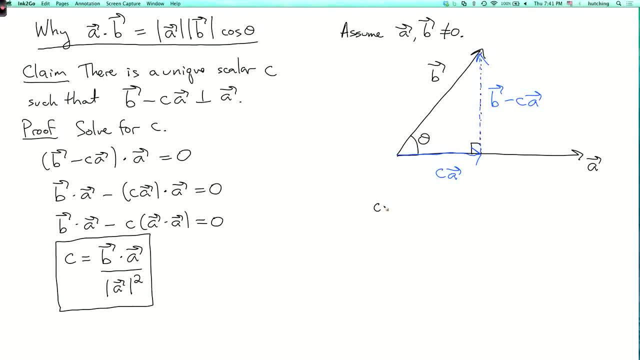 Well, what is the cosine of theta anyway? So the cosine of theta is the length of this adjacent side of the triangle divided by the length of the hypotenuse. So it's the length of c a divided by the length of b. That's actually not always true. 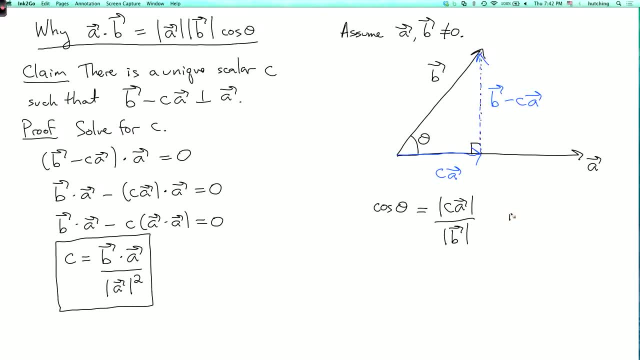 It's true when the pictures are shown, when c is bigger than 0. So if c is greater than or equal to 0. If c is less than 0, then the angle is going to be more than pi over 2, and the cosine is going to be negative. 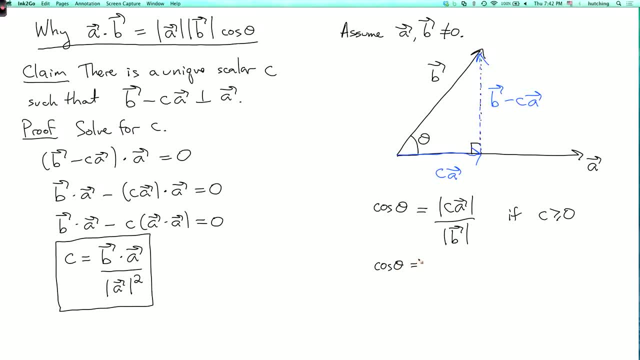 So the cosine of theta is minus the length of c, a over the length of b, if c is less than or equal to 0. And we can combine these two equations into one equation. by writing it like this, We can write: cosine of theta. 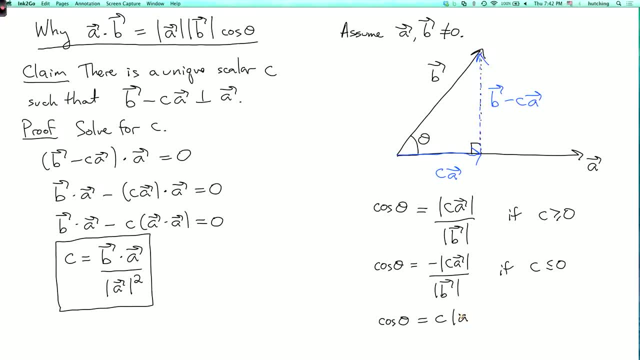 Cosine of theta equals c times the length of a over the length of b, And this is true both when c is positive and when c is negative. All right, now we're almost done. So now we combine these two boxed equations. So I'm going to take my equation for cosine of theta and plug in my equation for c. 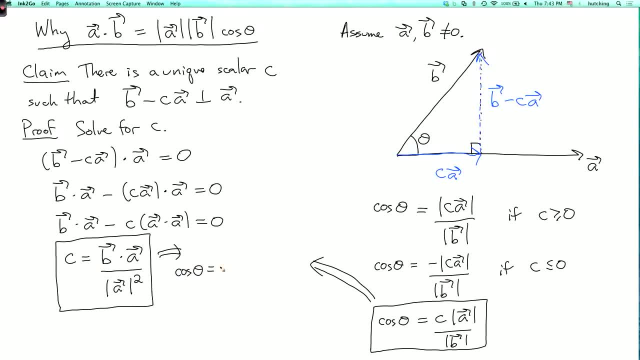 So I get cosine of theta equals So c here. So c here is b. dot a over the length of a squared And then I multiply by the length of a over the length of b And now I can cancel out the length of a here and cancel out this squared here. 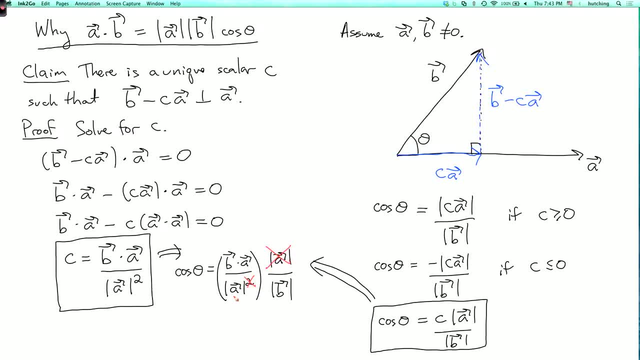 So I get: cosine of theta is b dot a over length of a times length of b And dot product is commutative, so that's also a dot b. So if you just clear the denominator you get the equation we wanted. So that's the proof.